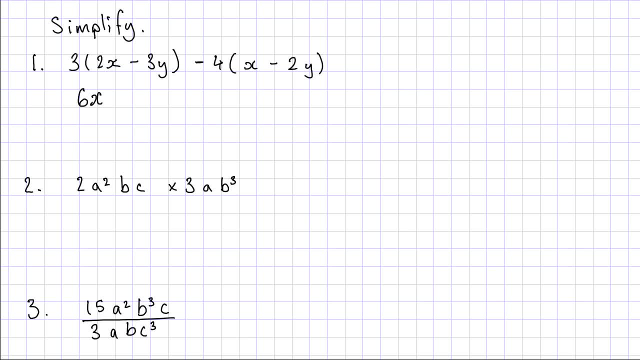 Then I'm going to multiply 3 by minus 3y, that's minus 9y. Now this is where I need to be a little bit careful. I need to multiply this minus 4 with the x, and I need to multiply the minus 4 with the minus 2y. 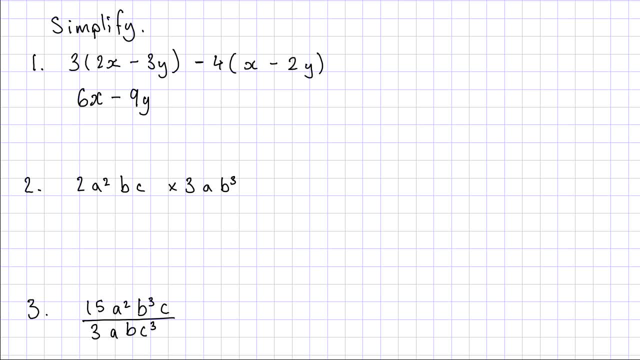 Now, it's very easy to make mistakes here, so we need to be careful here. Minus 4 times x is minus 4x. Minus 4 times minus 2y is plus 8y. Now this can be simplified further. 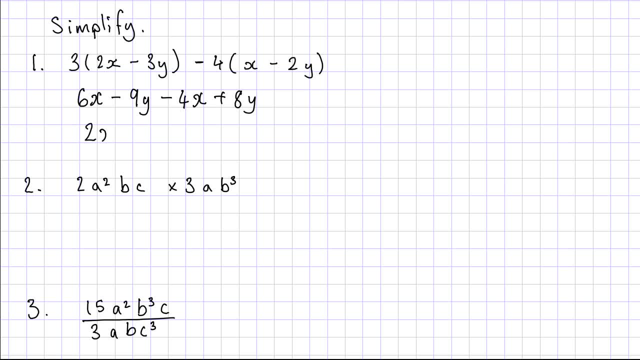 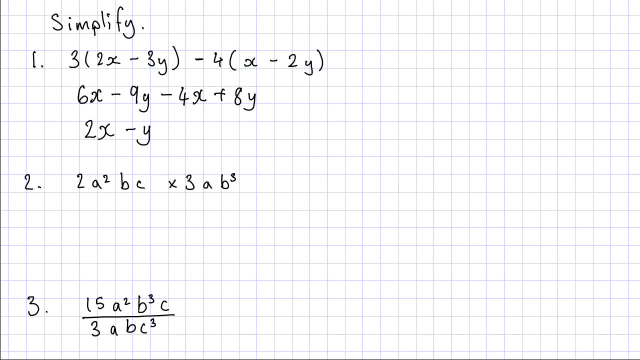 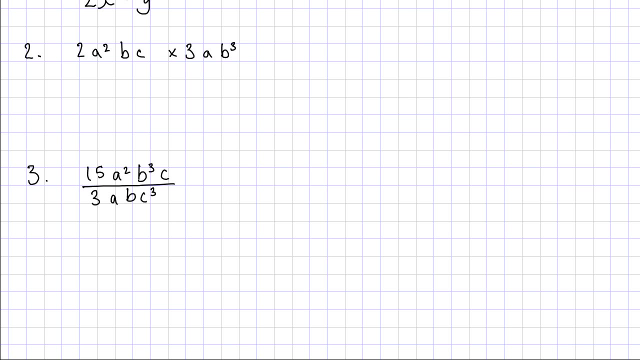 6x minus 4x is 2x Minus 9y plus 8y. 8y is minus y. Now the next question is a multiplication. Now I can change the order of multiplication and I will still be left with the same expression. 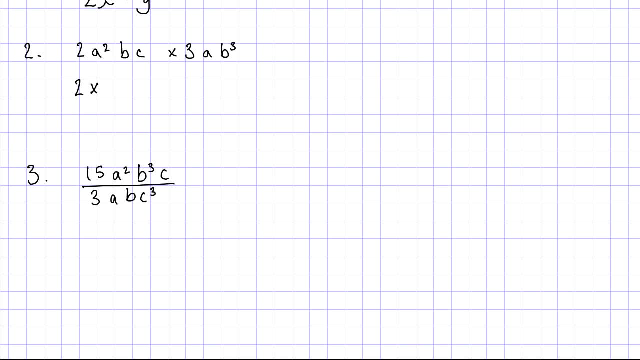 So I'm going to start by writing 2 times 3.. And then I'm going to say: times a squared, times a And times b, times b cubed And times c. So I'm just going to simplify it now. So 2 times 3 is 6.. 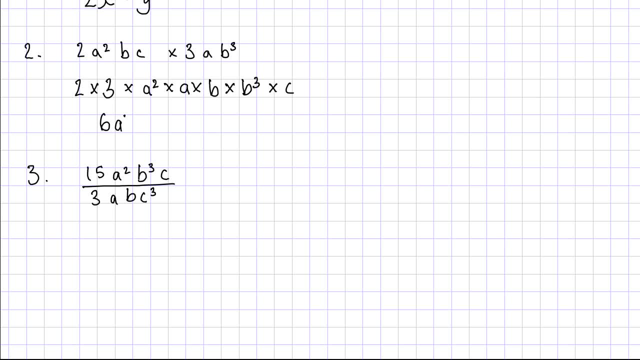 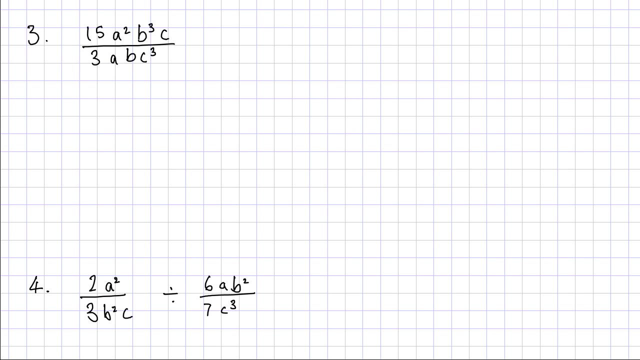 a squared times a is a cubed b times b cubed is b to the power of 4.. And times c, And that's the answer. Question 3 is a division. Now it's helpful to write this out as a product in the numerator. 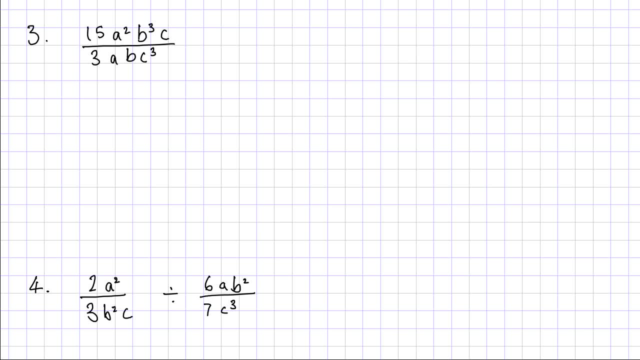 And a product in the denominator, And then it's easy to see what will cancel. So I'm going to start by writing 15 as 3 times 5.. a squared as times a times a, b, cubed is times b times b times b. 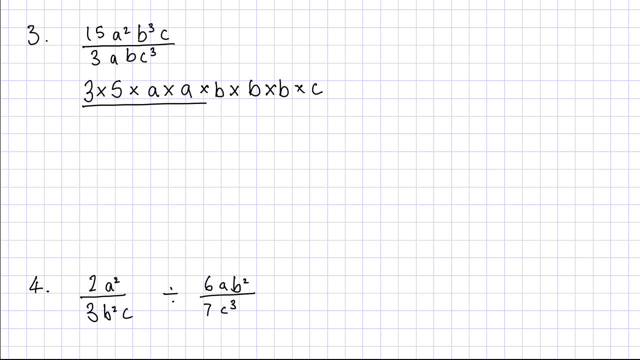 And then times c. All over 3 times a Times b, Times c. cubed is c times c, times c. Now I'm going to cancel things down. This 3 cancels with that 3.. The a cancels there.